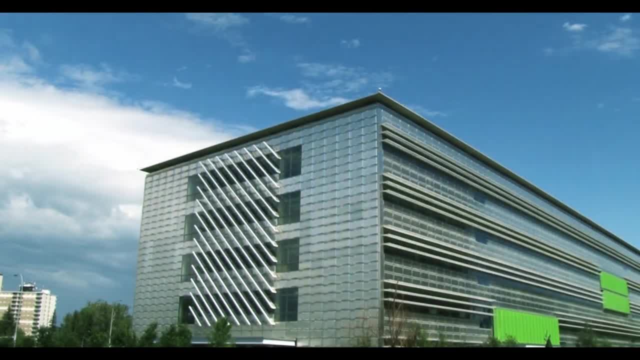 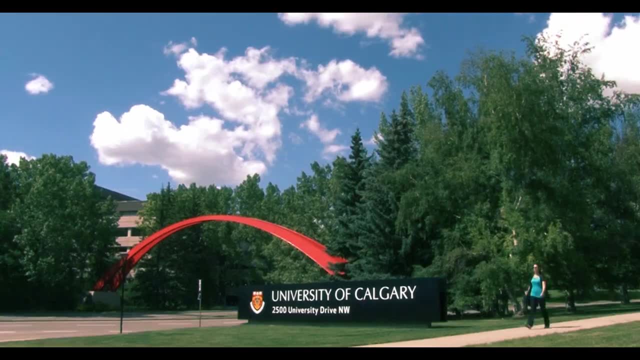 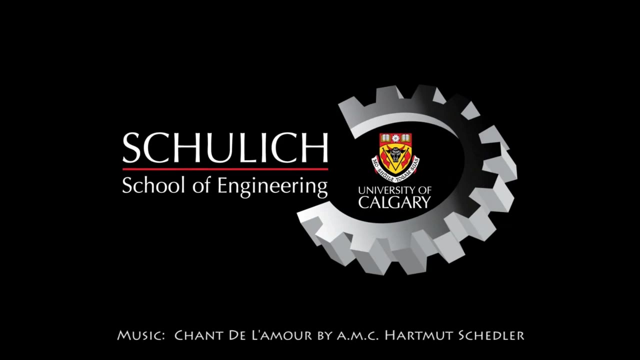 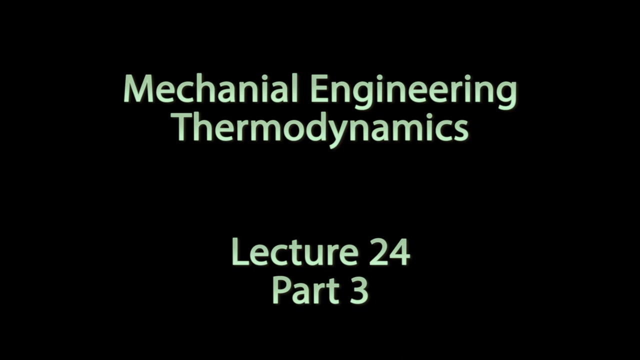 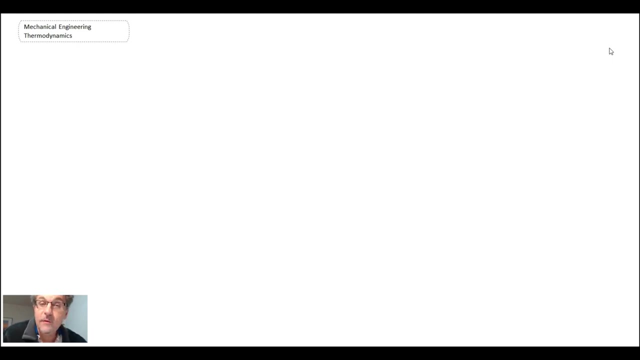 The next cycle that we're going to take a look at is actually quite clever from the perspective that it achieves similar performance to what we saw for the cascade cycle that had two different working fluids, yet it does this using only one single working fluid, And so this is multi-stage vapor compression. 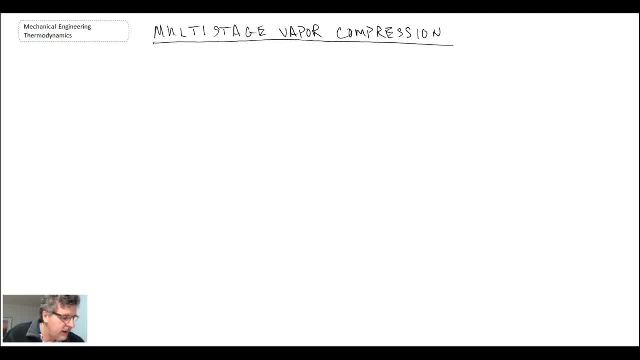 And in a way, it's similar to when we looked at multi-stage compression with intercooling for gas compression, But what we have here is a situation where the compressed refrigerant is lower than the atmospheric temperature. So the question would be then: how do you cool it? 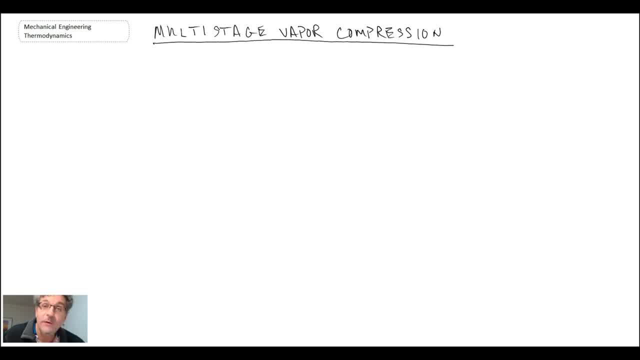 And the way that we'll cool it with a cycle is we mix it with refrigerant from another part of the cycle. It's kind of almost like a regenerative process that we looked at When we looked at other cycles earlier on in the course, both with Rankin as well as. 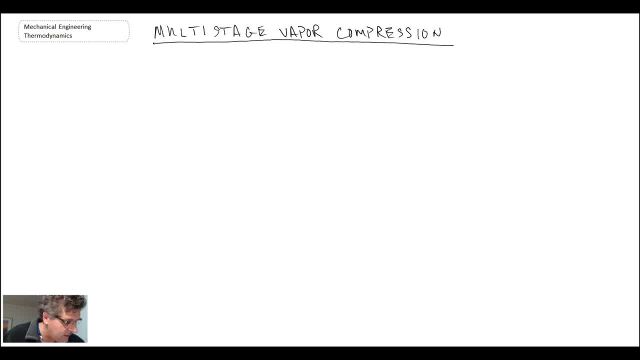 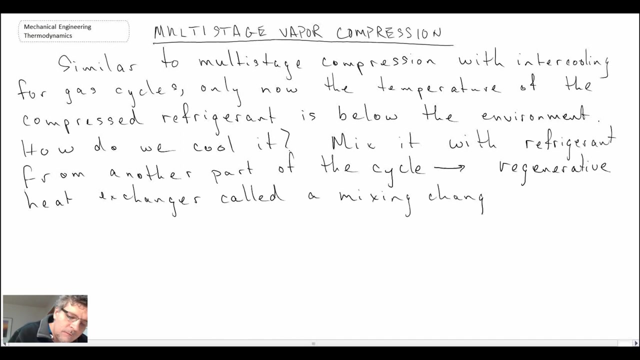 we looked at the regenerative when we looked at the Stirling cycle. Now, that was for a heat engine. This is for refrigeration. So what we'll do here is, in order to cool our refrigerant, we will be mixing it with refrigerant. 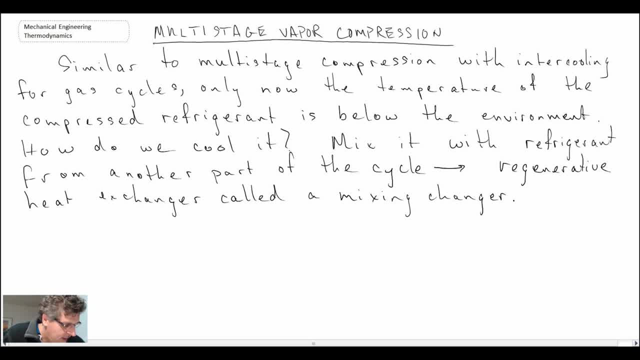 from another part of the cycle that's at a low temperature, And consequently, in a way, this is similar to a regenerative heat exchanger, although what we're using is just a mixing chamber, something that we looked at when we studied the Rankin power cycle. So let's go ahead. 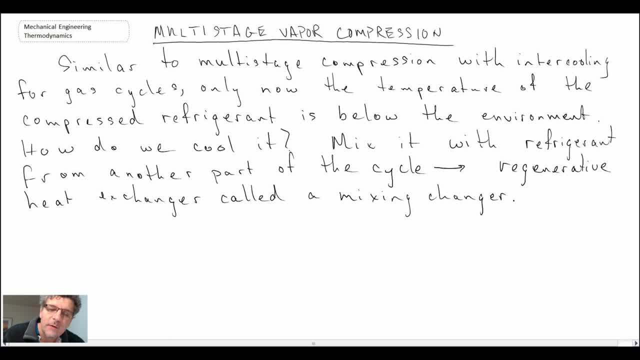 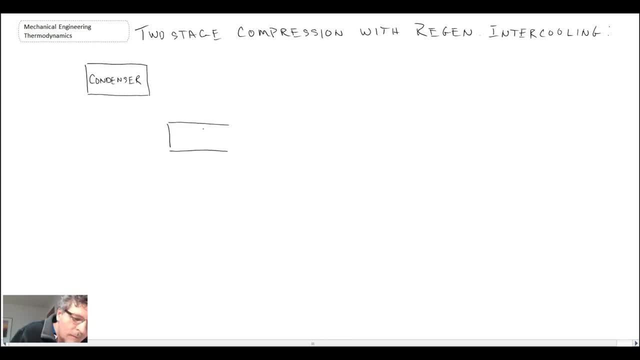 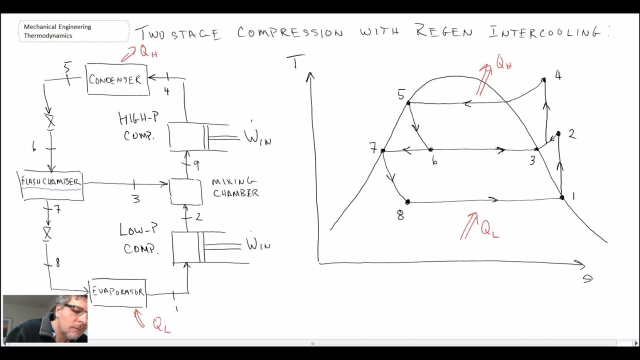 and take a look at this. We're going to look at it for a two-stage compression process. So we're going to take a look at it for a two-stage compression process. So there is our schematic as well as diagram for the two-stage compression refrigeration. 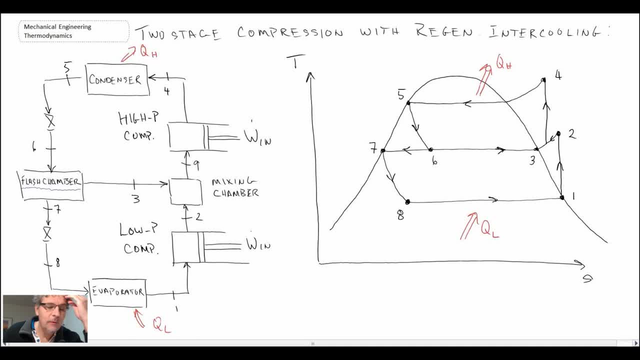 system And one thing: well, what's happening here? The biggest change would be, you'll notice, we have this flash chamber And basically this is a device that can separate a multi-phase fluid, Because we have a multi-phase fluid coming out after our condenser. We're at state six, which 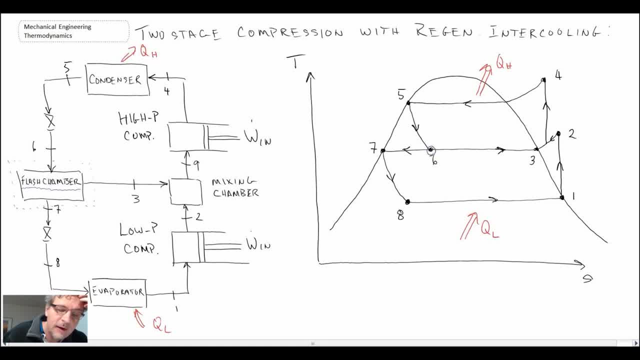 on our TS diagram is right here And what we are doing is we're stripping out the vapor And the saturated vapor is what is at state three. So on our TS diagram that is there And that is then what flows into the mixing chambers. That's the vapor at state three there. 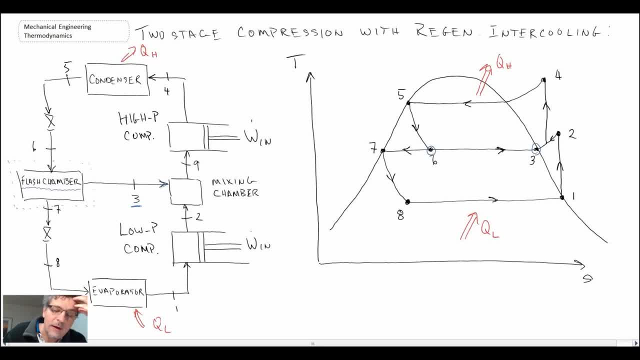 The percentage of vapor that is going two, three is equal to the quality of the refrigerant after the throttling process from five to six. So we can say the percentage going to three is X- six. And if we say that the remaining the liquid is stripped off And it goes to state seven down to one, 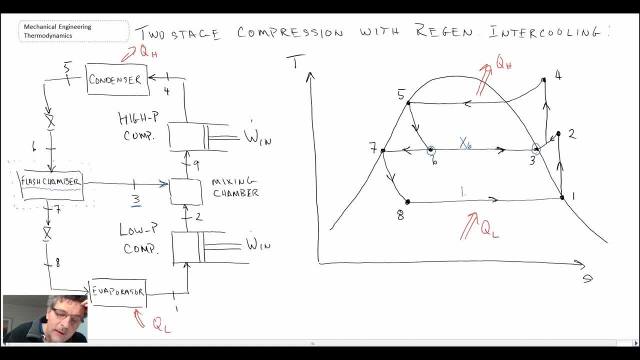 or to eight and then over to one, So we can write the percentage of liquid or fluid going there through the condenser. sorry, the evaporator at the bottom of the cycle is one minus X six, And so we break the fluid in two So we have a hundred percent of. 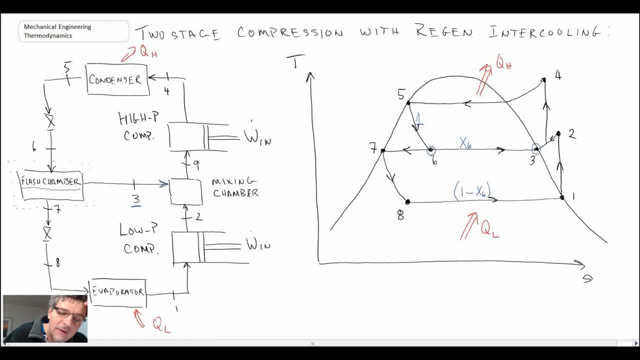 the fluid coming through here, And once we get to six we take X six off and that goes to three, and then one minus X six goes to seven. And that is one of the different components, the liquid that's going to go into the Rails and then that goes to the liquid. So we have to do that. 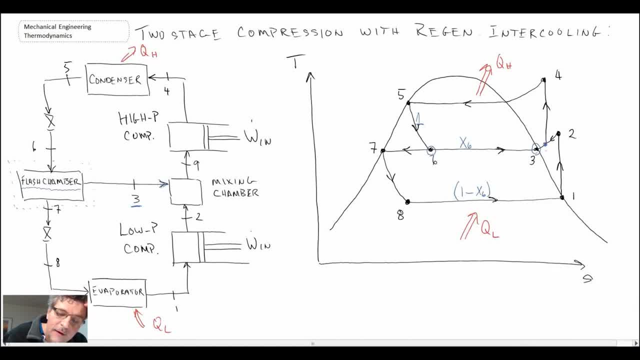 So the second thing is, what we're going to do is we're going to change the state nine from state three and then we're going to change the state nine. we're going to change it to state nine and then we're going to take the liquid from state three, mixing it with fluid at state two. 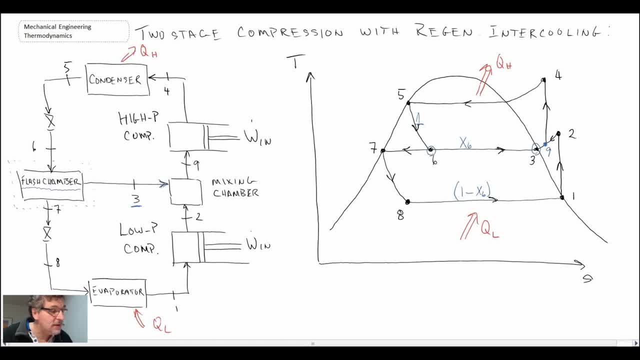 and we end up at state nine, which then goes into the high-pressure compression process. So that is the two-stage compression refrigeration process. I'm going to stop here if I'm going to continue refrigeration cycle. What we'll do now is we're going to take a look at the first law applied to 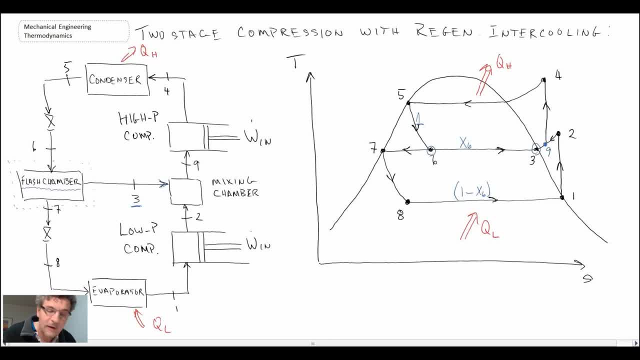 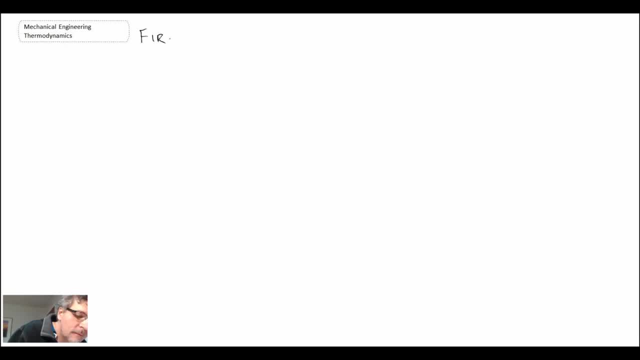 the mixing chamber and we'll see what the equations bring by doing that. So let's take a look at the first law. So, for the mixing chamber, what we can say is that it is adiabatic and that there is no work being done. 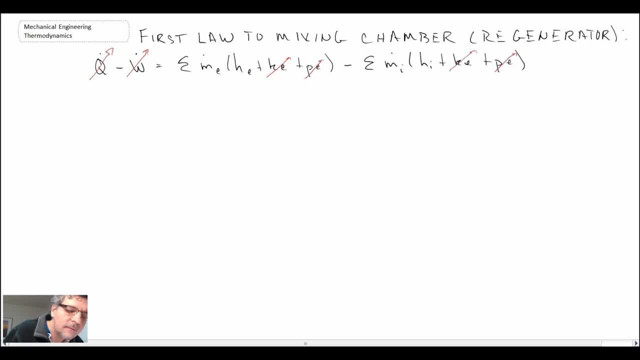 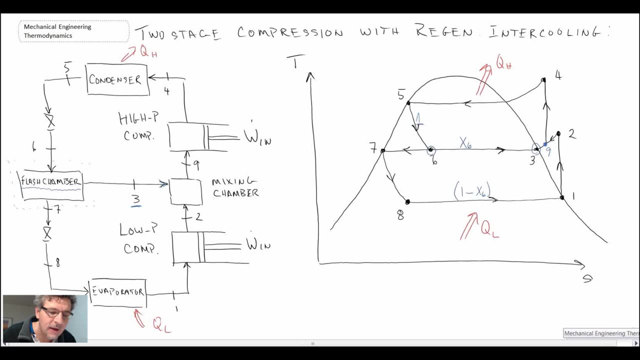 We neglect kinetic and potential, And that's the first law And that's the second law. So that's what we end up with When we look at the mixing chamber, we have fluid at state 3 coming in, fluid at state 2 coming in and then fluid at state 9 leaving. 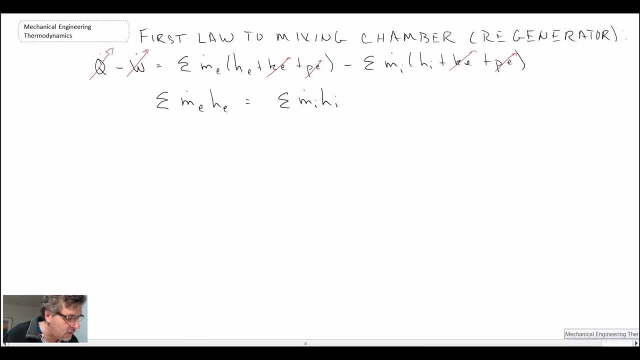 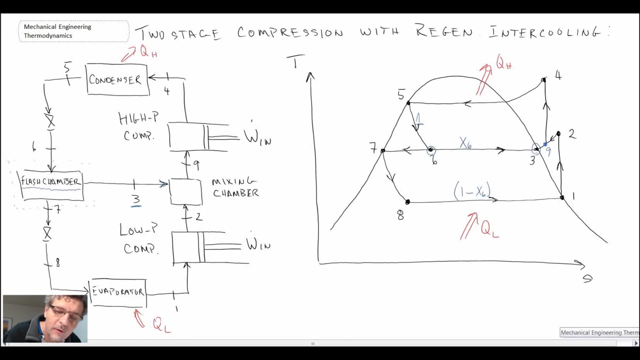 So that enables us then to figure out what's coming and what's going. So the fluid leaving is fluid at state 9.. And what's coming in is state 3 plus state 2.. Now, in order to determine m.3 and m.2,, looking back here we have 100% mass flow is going through state 4, 5.. 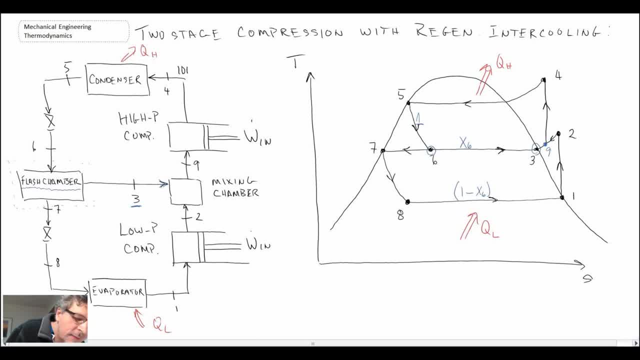 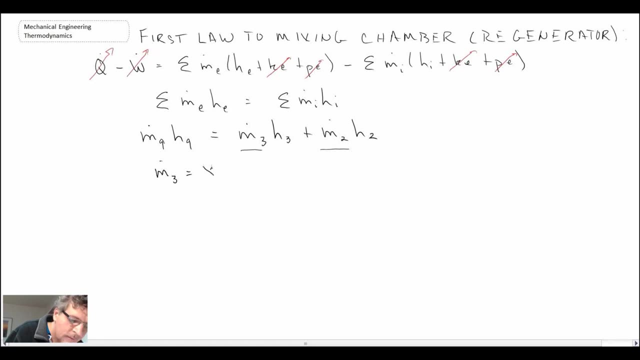 So up here we have 100% mass flow. The other streams, the mass flow is lower. so we need to acknowledge that. when we're looking at this Now for m.3, it is x6, which was the quality at the end of the throttling process times- m.9.. 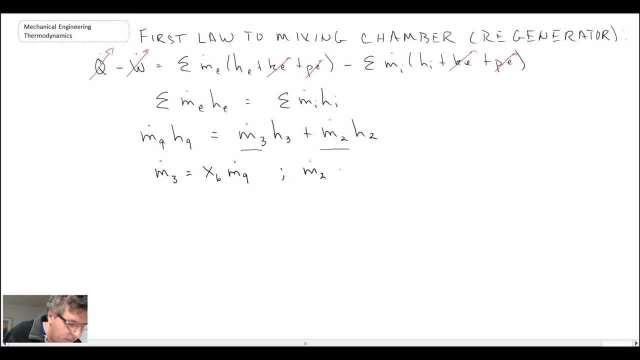 And if we say that, then m.2 is 1 minus that. So that enables us to determine the mass flow rate for 3 and 2.. We can then plug in for the enthalpy at state 9 and obtain the mass flow rate for 3 and 2.. 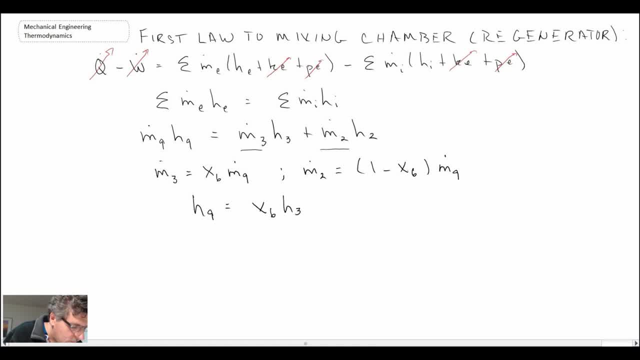 So that's the same of the following And that's an equation that we can use then for our mixing chamber or regenerator and determining the enthalpy at state 9.. Other things that we would do: we would want to be able to get the coefficient of performance. 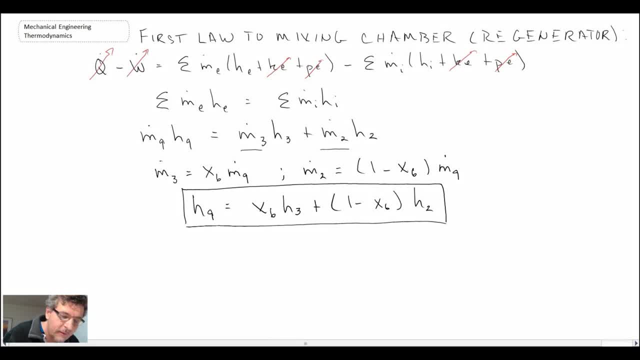 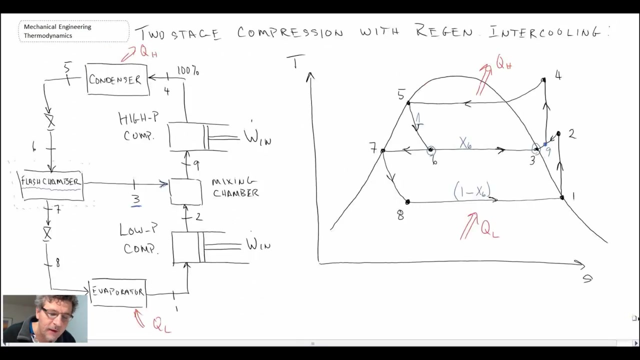 And so we would look at the low temperature heat transfer coming from our low temperature source, whatever we're trying to cool, and then expressing that in terms of mass flow rate. And we have to do this because we do not have 100% of the mass flow rate going through the 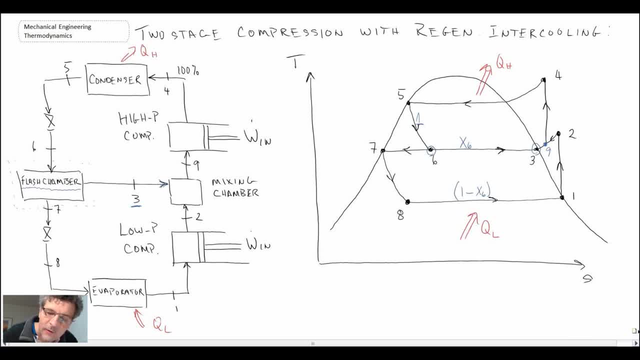 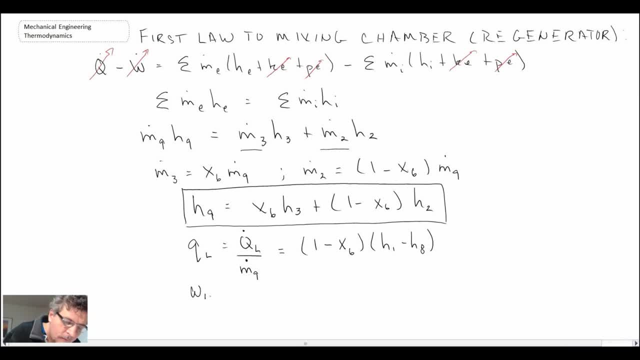 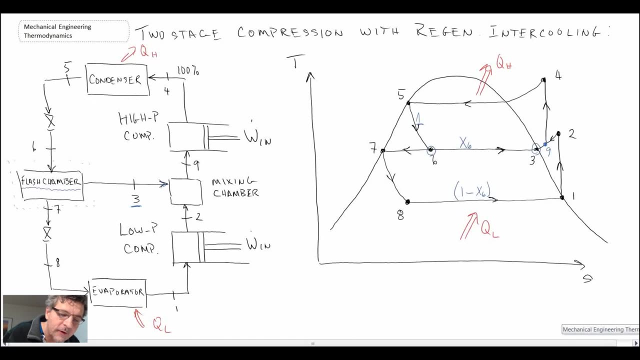 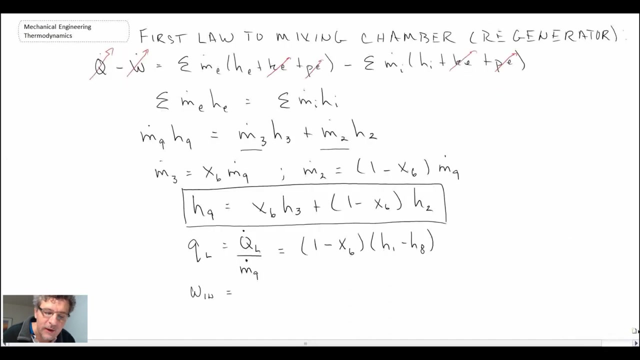 evaporator, We have 1 minus X6 going through. As for work N, we will have different mass flow rate going through the low pressure compressor versus the high pressure compressor. High pressure compressor will have 100%. the low pressure will have 1 minus X6. We need to acknowledge that as well. 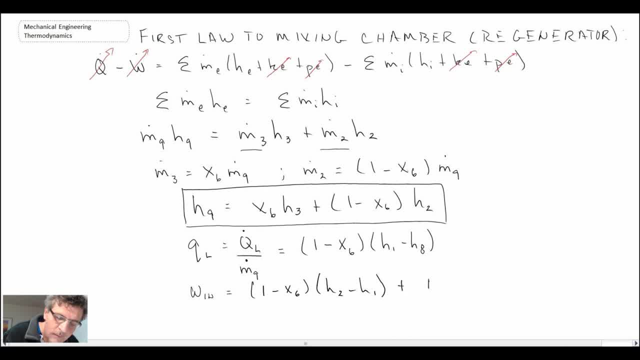 So that's where you have to be a little careful with the work, as well as the heat transfer. Once you've done that, you can then determine the coefficient of performance in terms of mass flow rate 9.. And so that would then be a way that you could determine. 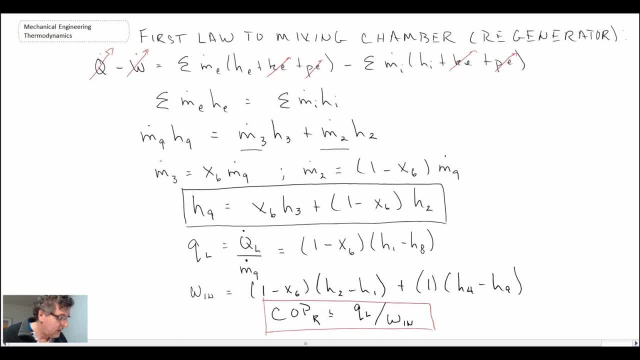 the coefficient of performance for this multi-stage vapor compression cycle.